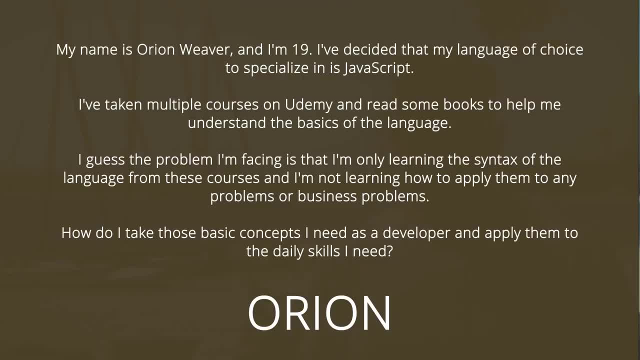 I've taken multiple courses on Udemy and read some books to help me understand the basics of the language. I guess the problem I'm facing is that I'm only learning the syntax of the language from these courses and not learning how to apply them. 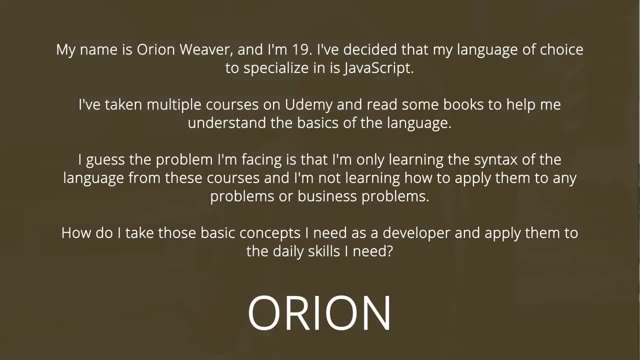 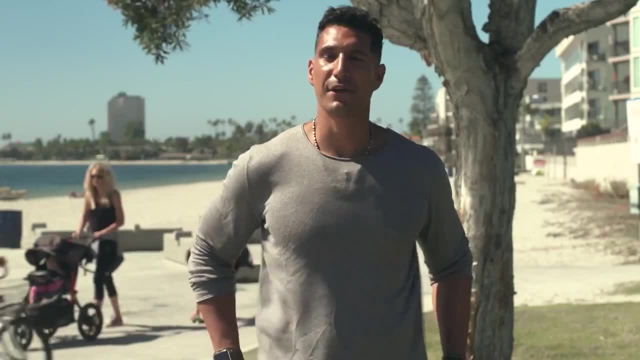 I don't want to come to any problems or business problems. How do I take those basic concepts I need as a developer and apply them to the daily skills I need? Like I said, straightforward, simple, simple answer here. I'll tell you what you do, my friend Orion. 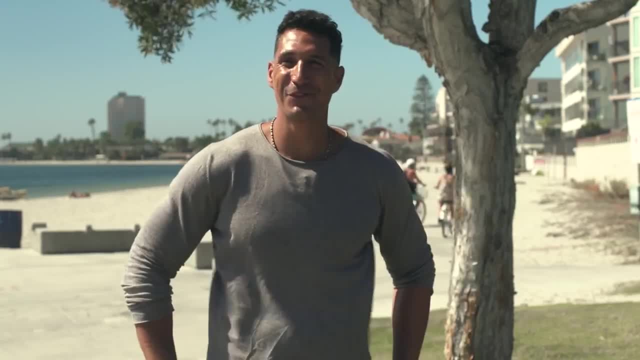 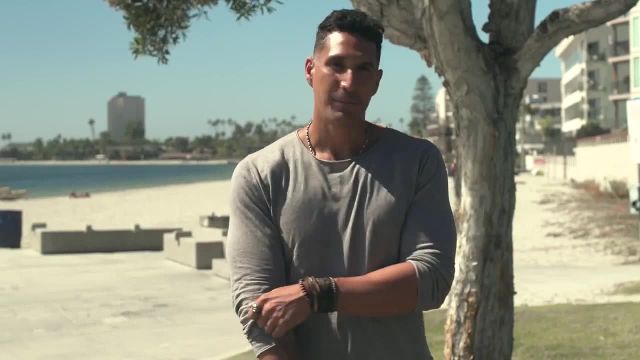 You build something. I know it's uncomfortable and it's just so much easier to just take a course and learn the thing or read a book, but you got to build something, my friend. That's what you got to do and you got to struggle through it. 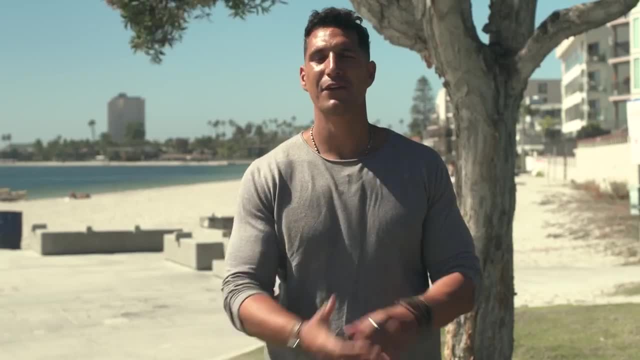 It is. It's going to be painful and you're going to be like I don't know what the fuck I'm doing. You're going to be like I don't know if this is worth it. What am I doing? This is crap. 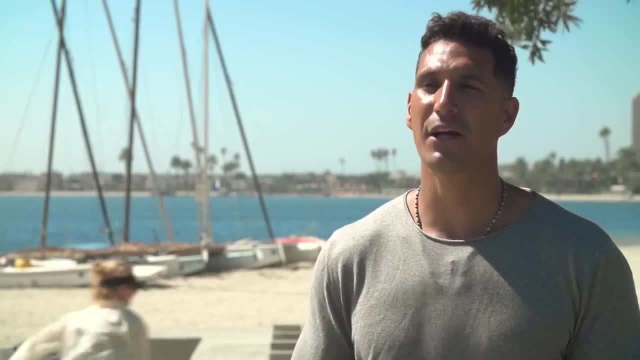 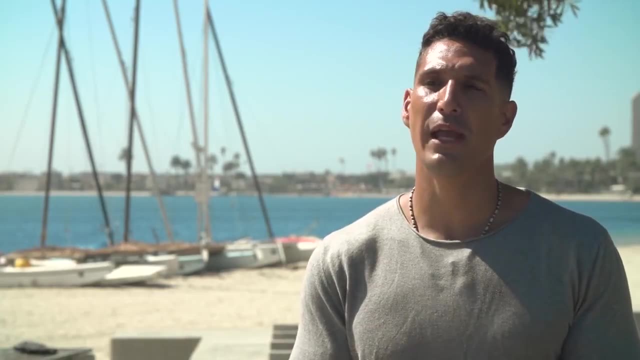 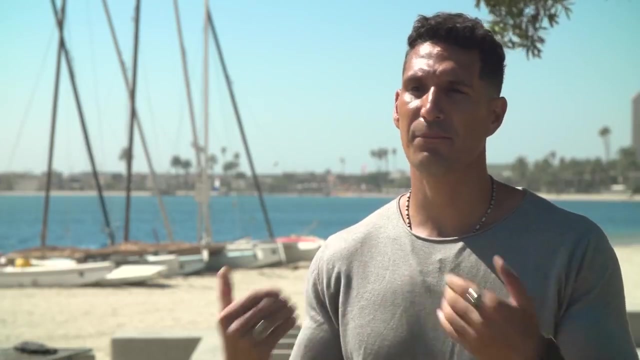 That's how you grow. You grow through being uncomfortable in life. This is simple. Like I said, what I want you to do is I want you to go, and I'll make this real simple for you, because I like to separate the process of creation from the process of building. 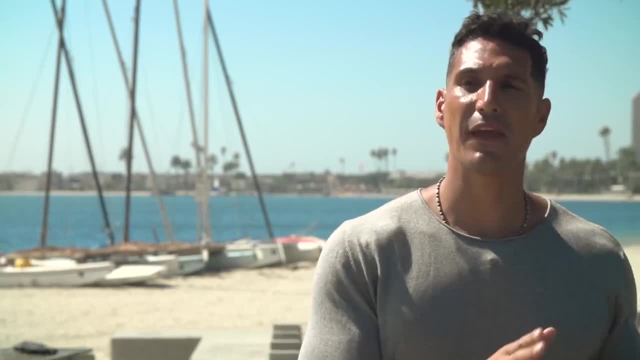 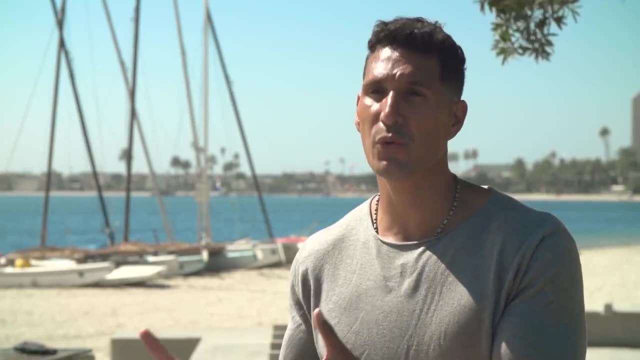 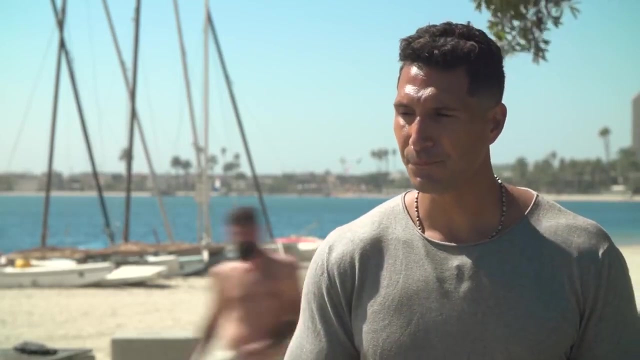 because creation and creative work is one thing, and that is— It's difficult in itself, but then actually like the construction of learning how to use your tools is another thing. I could give you an analogy, maybe from woodcrafting or furniture- Actually, from all—a lot of artists did this. 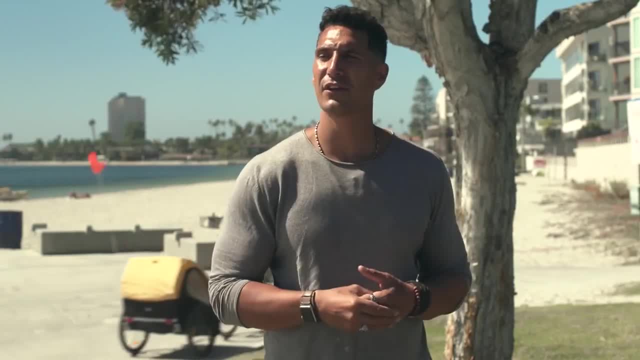 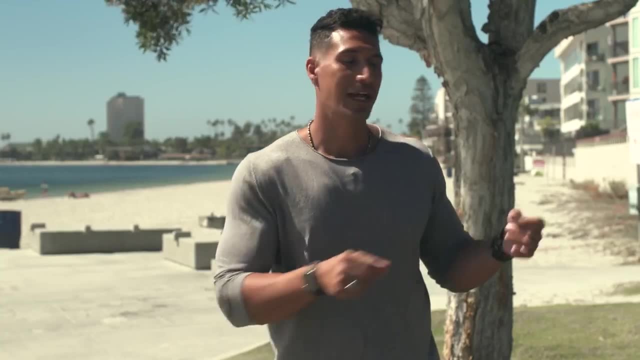 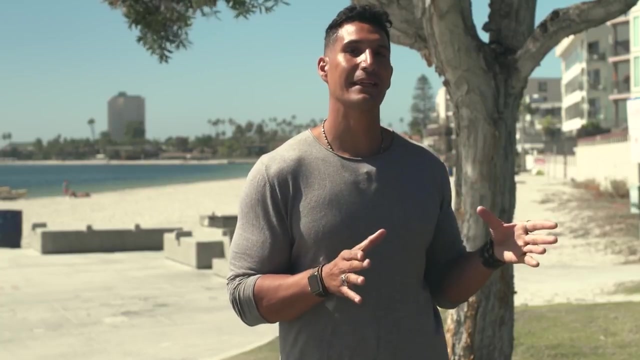 He didn't just start painting his Van Goghs. What he did is he started painting other—he copied other people's art- the masters, like the other artists- and he just tried to duplicate it. That allowed— That allowed- him to develop his technique, his skill for painting- not creative at all- 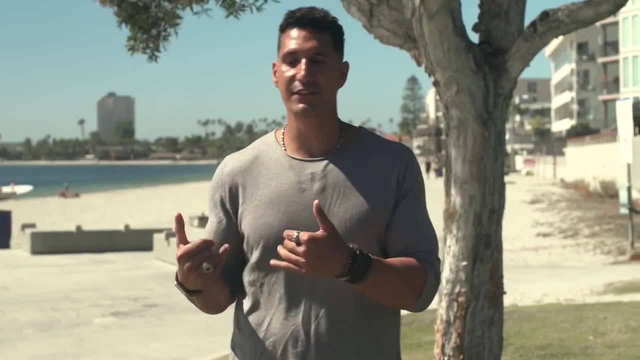 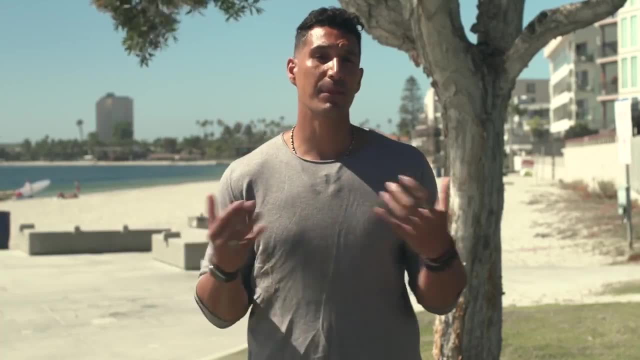 It's not creative at all. But once he did that and he developed that skill, then he started painting his own paintings. A lot of artists did this, A lot of sculptures did this. A lot of people do this today. You should do this. 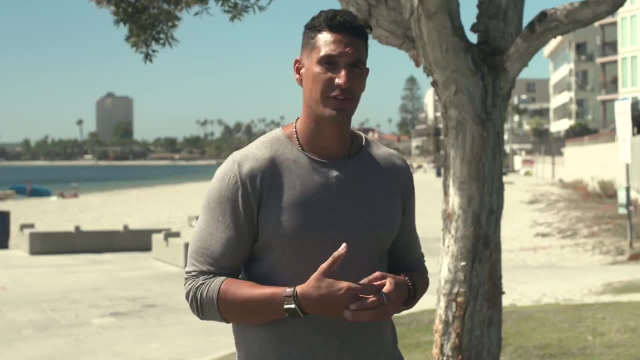 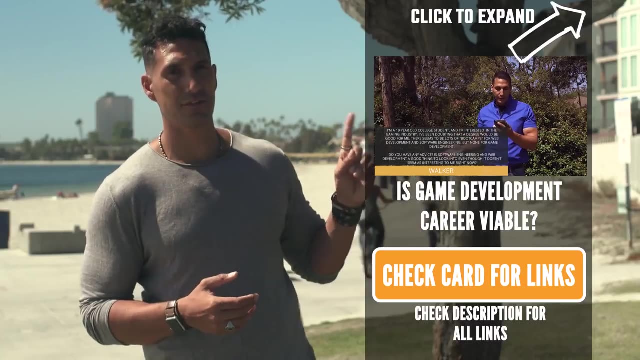 What do I want you to do? I want you to go and I want you to look for some application out there that already exists If you want to be a game developer. I've done some videos on game development and I think I've given this exact advice. 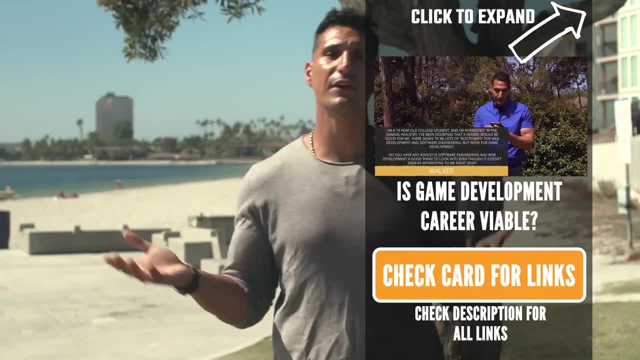 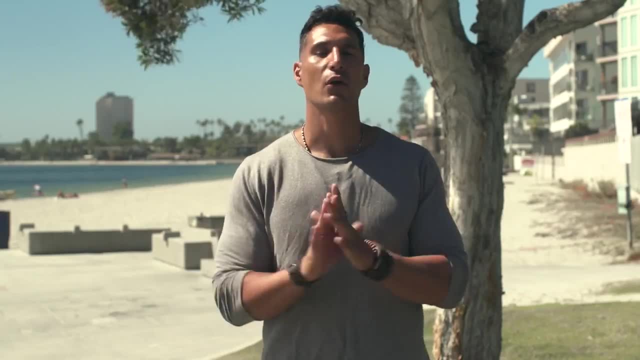 You can check that out. I've probably got a playlist there. Then go find a video game like Pac-Man or something simple and just copy it. I just want you to make a perfect clone of it. I don't want you to try and innovate or do anything unique. 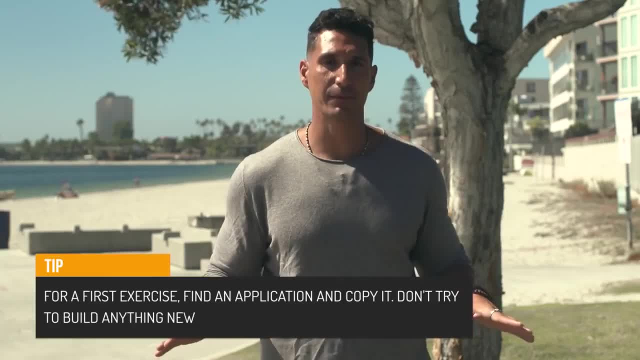 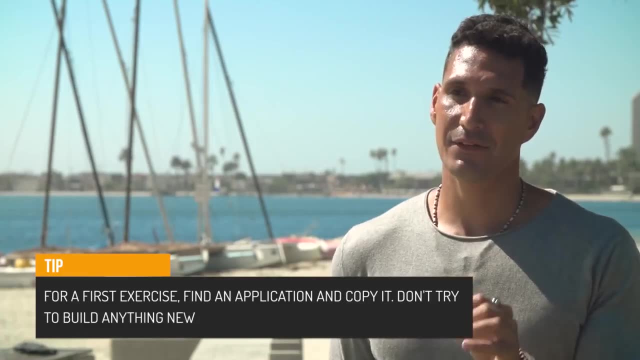 I just want you to make it as true to the original as possible. Same thing if you pick a web app or you pick an app on a mobile phone. Why? Because that is what's going to get you the skills. It's like the artist learning how to use the paintbrushes and using the paints and making the colors. 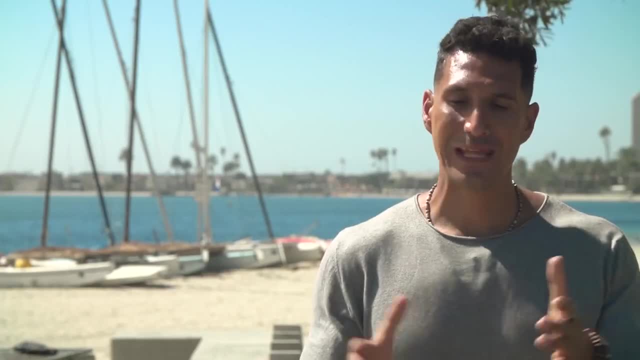 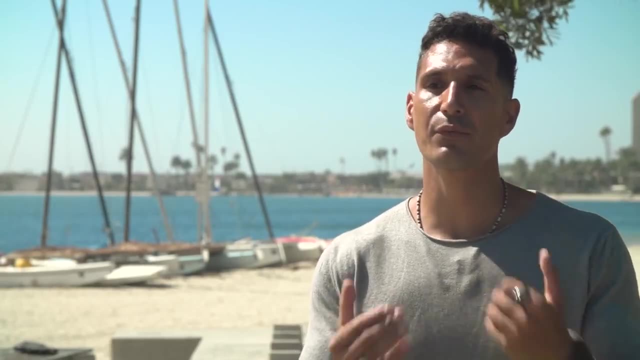 It's the same thing. It's the same thing That's going to take you from— It's going to take you from this book knowledge to an actual application knowledge, and it's going to take out the creative element, which you would struggle with, because it's really really hard to do both at the same time. 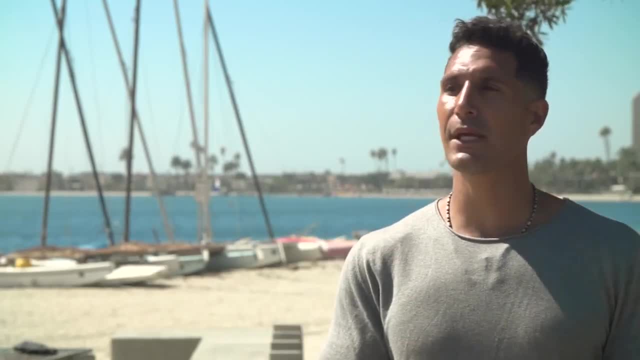 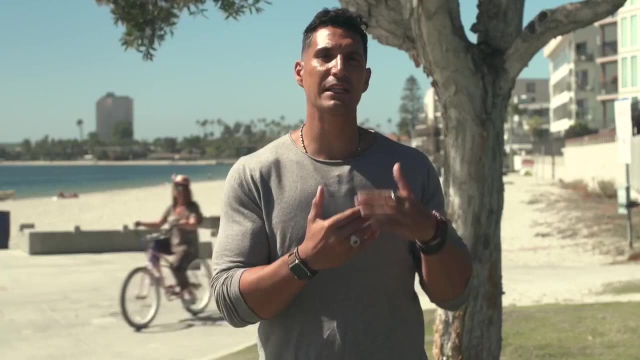 Now, once you have that ability, you duplicate a bunch of apps. You say, okay, I want to create a to-do list app. I want to create, like, a Gmail clone or whatever it is. Pick the complexity of the app that suits where you're at. 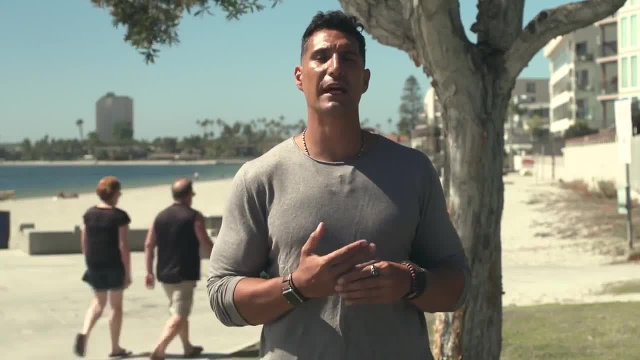 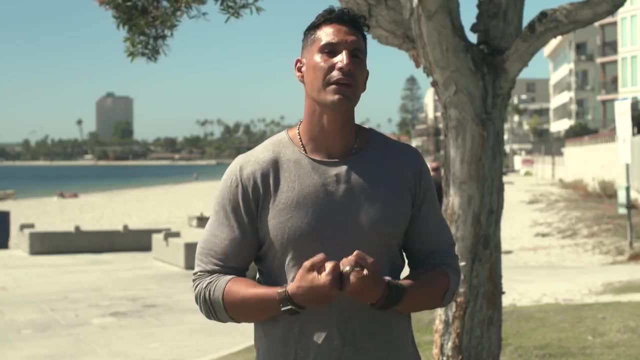 Pick something simple to start with. Then, once you've done that quite a bit, then you will have the mastery of the tools. Once you have the mastery of the tools and the application of those tools, then you apply some creativity. Then you say, oh yeah, I want to create an app that does this. 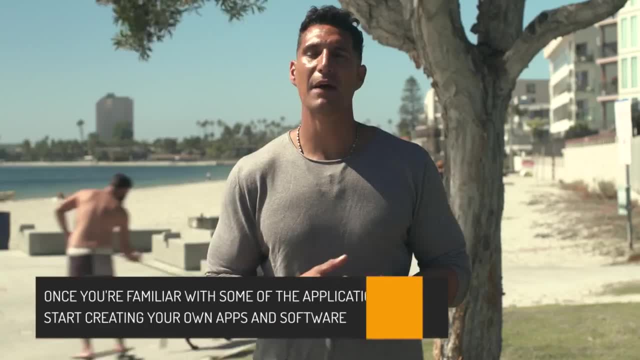 and you design the app or you design the thing, and then you can make that happen. Then also, when you're in the real world and you're working on something and someone gives you some specs and they say, hey, can you create an app that does this? 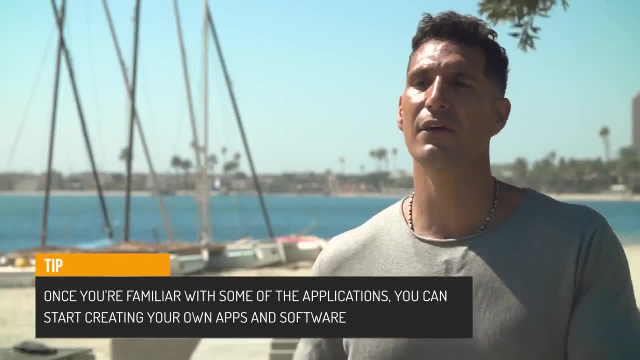 They tell you—you say: well, what do you want it to do? You say: oh, yeah, yeah, yeah, I can do that. I know other tools. You just tell me what you want and then I'll build it for you. 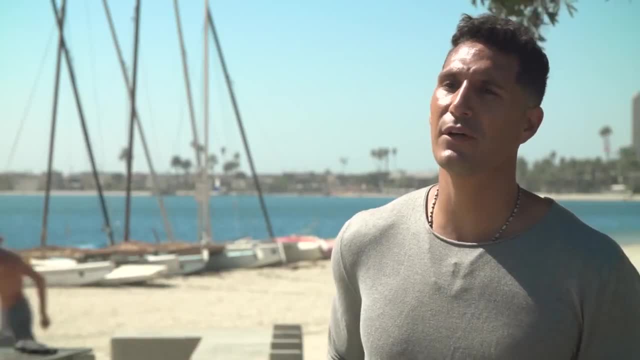 You see what I'm saying. This is my best advice on this. Like I said, real simple, Real simple question. I mean real simple answer here. but you've got to start building. The best way is just to duplicate something that already exists. 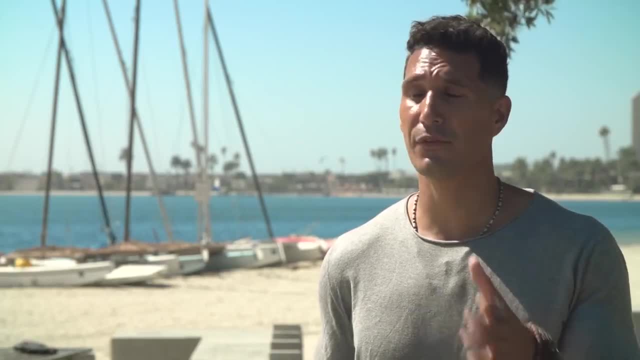 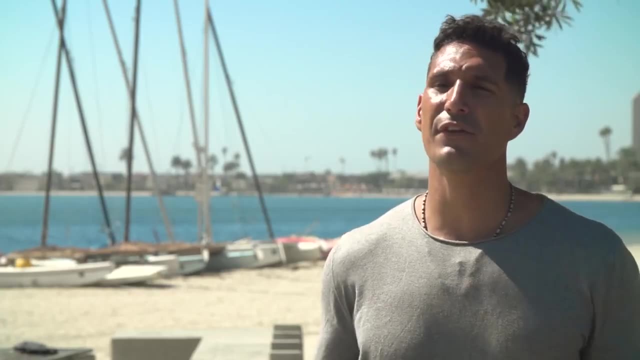 When you do that honestly, you'll become a master of the tools and you'll feel super confident. by doing that, So many developers, you need to listen to this advice and do this, because you're struggling, You're fighting. You think you're going to learn everything from a book or from doing tutorials. 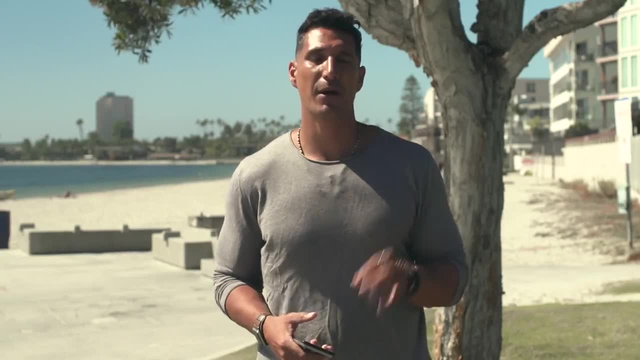 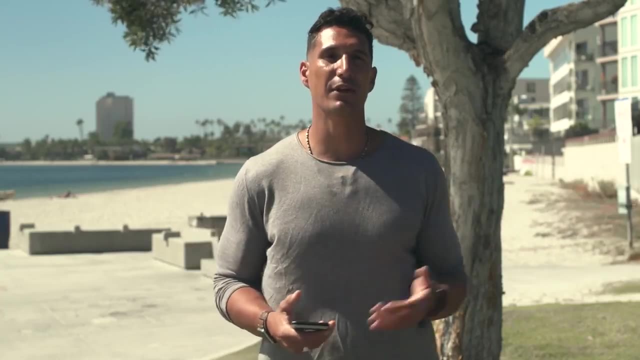 It's not going to happen. You've got to actually apply it. Like I said, don't waste the time of trying to come up with a creative— It's hard enough to create, It becomes—. You've got to become creative and instead duplicate something that already exists.